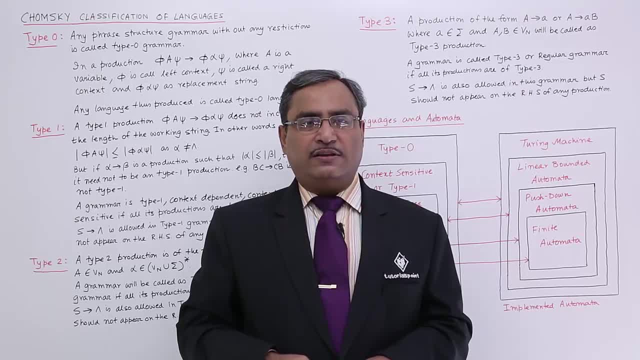 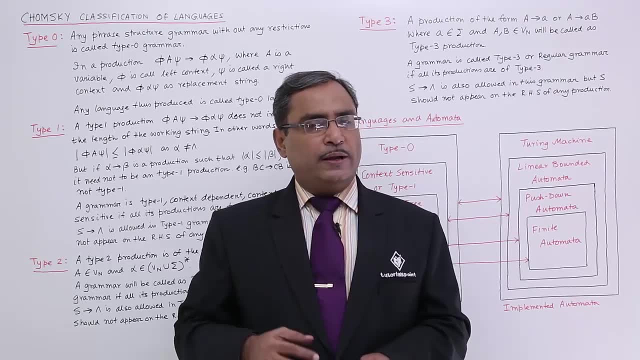 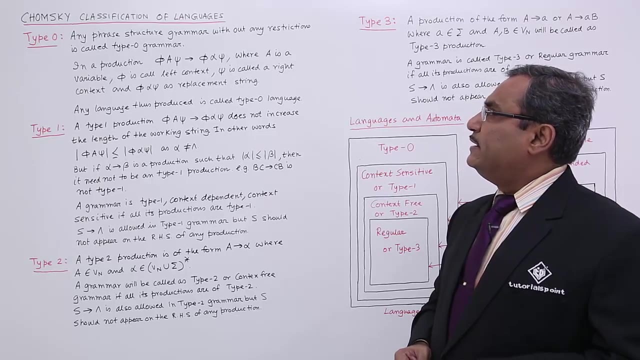 In this session you are going to discuss Chomsky classification of languages. We will be having four classifications: type 0 to type 3.. So let me go with the type 0 at first. See: any phrase structure grammar without any restrictions is called type 0 grammar. So any grammar will be. 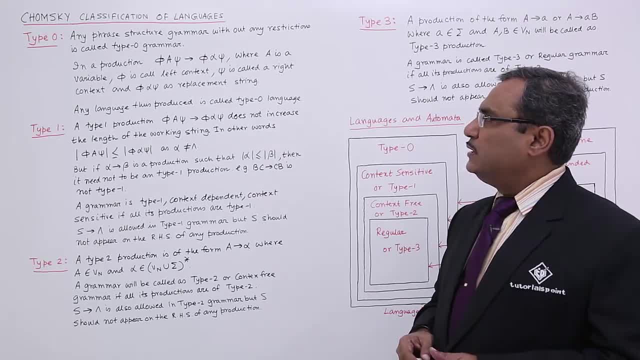 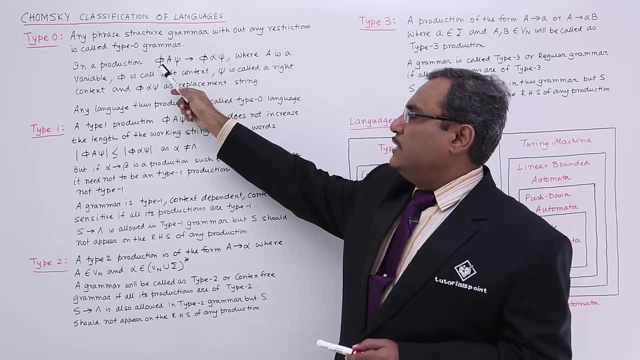 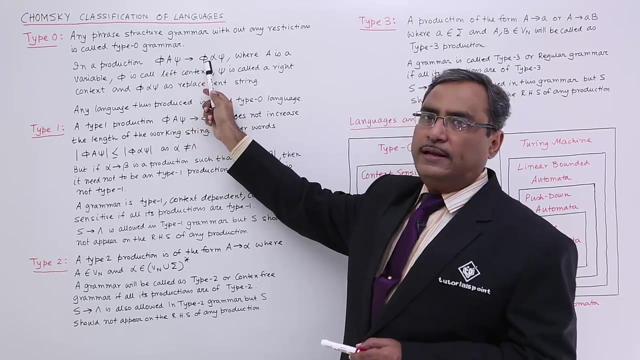 falling under the category of type 0. In a production there is a phi a xi produces phi alpha xi. look at this very very production. this phi is unaltered and this xi is also unaltered. on the left hand side they are existing and also on the right hand side. Here a is a variable, here is a. 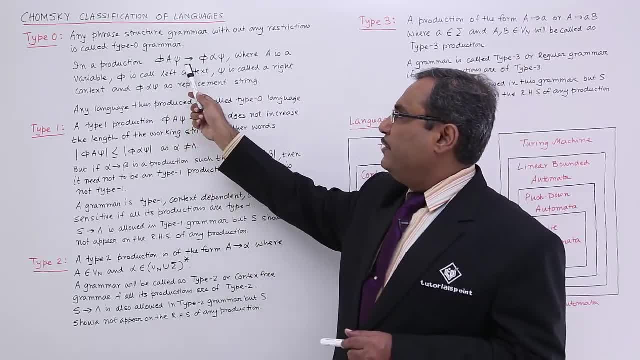 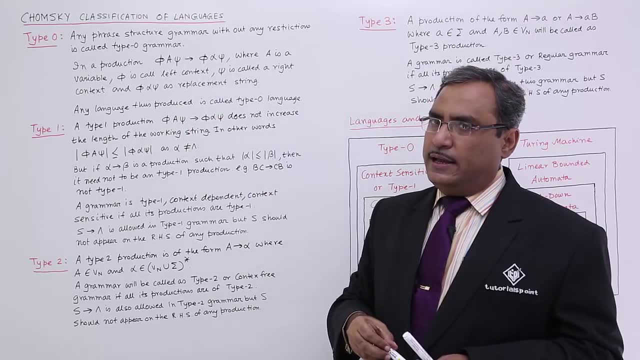 variable. variable means, you know, there is a non-terminal and it has been written in capital letter. that is why So phi is called the left context, as it is on the left hand side, and then xi is also known as the right context. So it is the left context and is the right context. 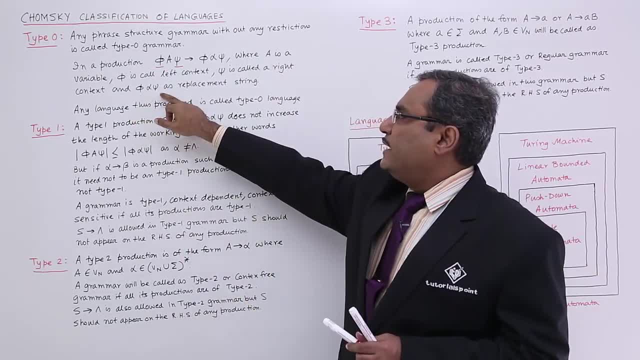 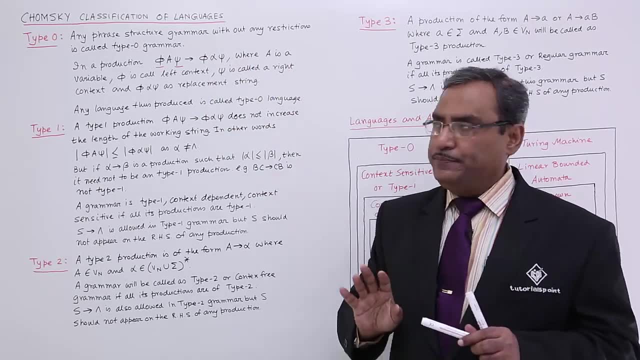 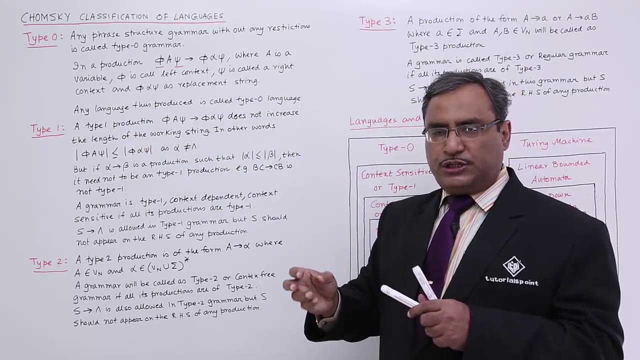 And that is a phi alpha xi as replacement string. So that is known as the replacement string. So this is my type 0 grammar. Any language thus produced is called type 0 language. So using type 0 productions, using type 0 grammar, all the languages, whatever will be produced, will be. 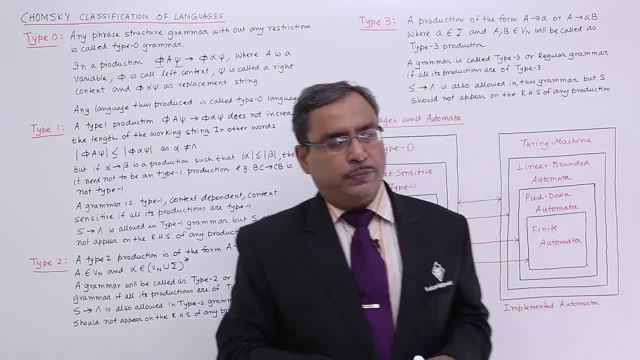 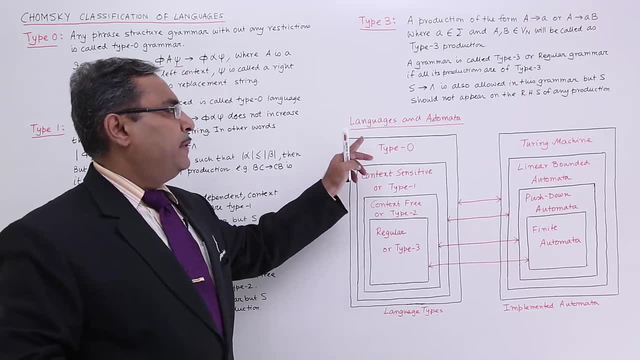 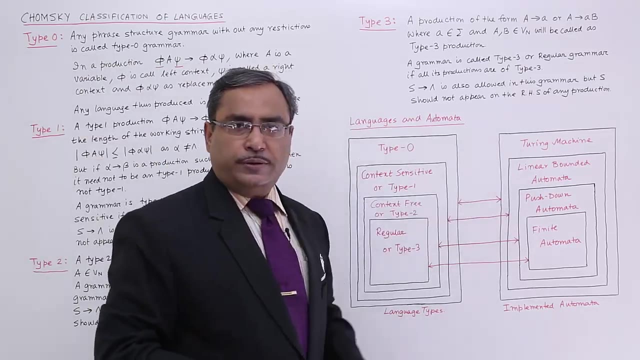 known as the type 0 language. So we have completed type 0.. Now see here: type 0 is the superset. This is the superset. So this is that my type 0 language and the respective implementation will be your Turing machine. So what is the Turing machine? How does it? 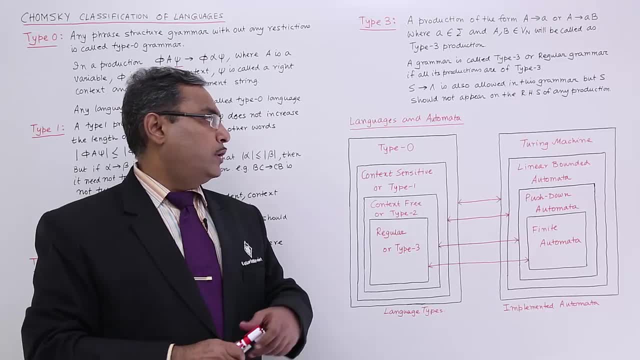 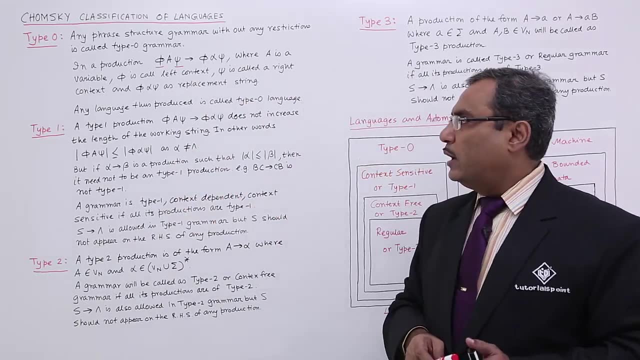 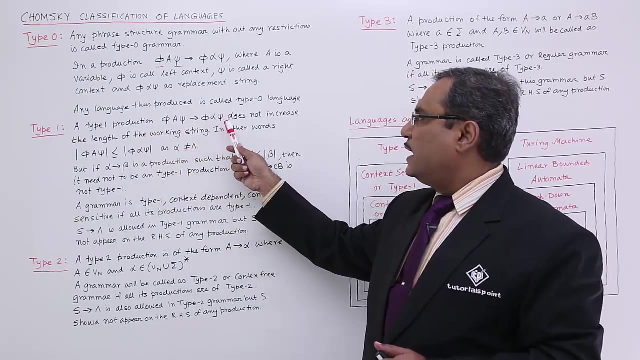 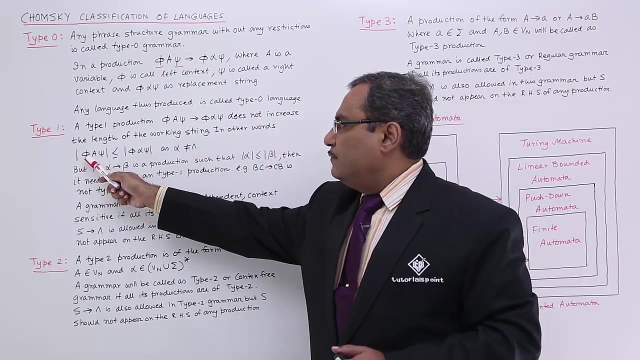 operate. We will be discussing that one in the later videos. So type 0 is actually corresponding to Turing machine. Now let us go for the type 1.. A type 1 production, that is, a phi a xi, does not increase the length of the working string. In other words, that means phi a xi. 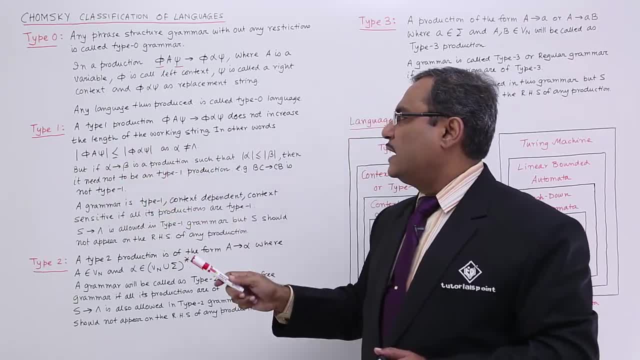 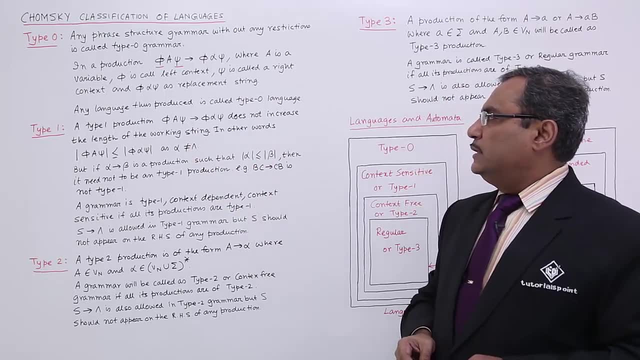 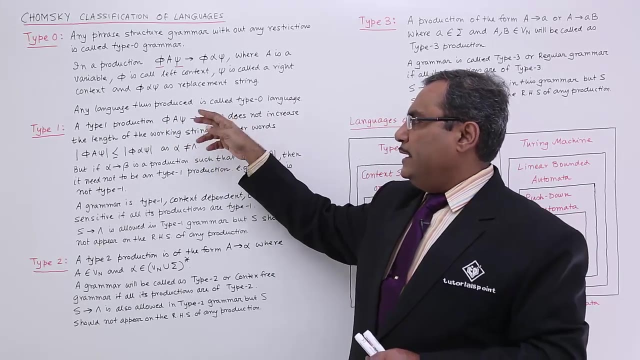 its length must be less than equal to phi, alpha xi, as alpha is not equal to kappa. Now the thing is that let us suppose this is my left hand side of the production. This is my right hand side of the production In case of type 1 production, always the right hand. 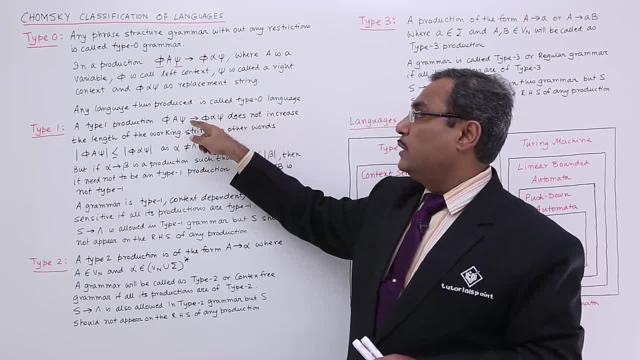 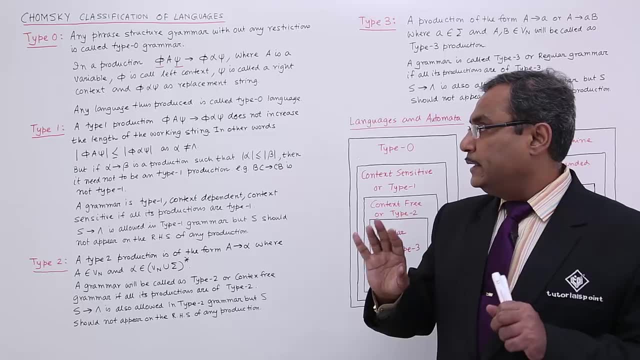 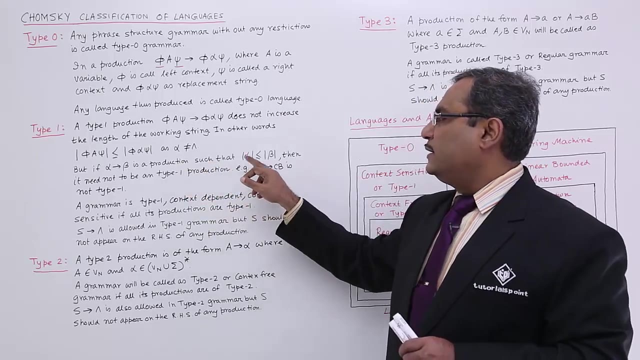 side, its length must be greater than or equal to the length of the left hand side. So that is only one constraint in type 1.. So but if there is a production called alpha produces beta, is a production such that length of alpha is less than equal to length of beta, then 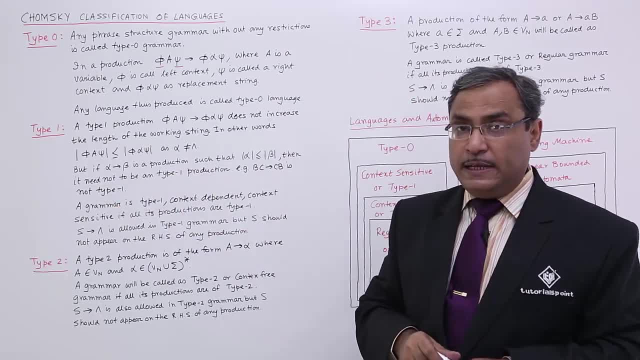 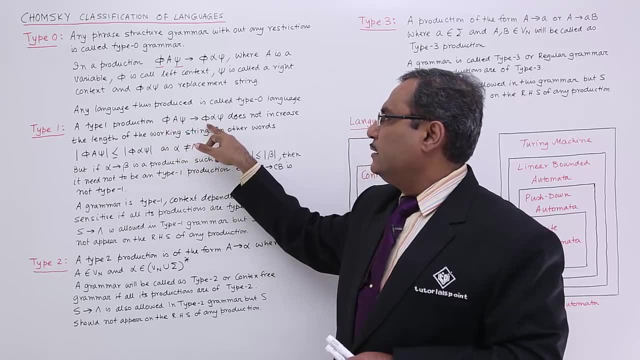 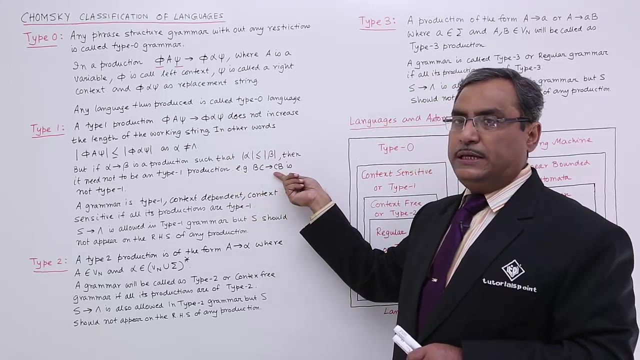 it need not to be a type 1 production. That means you should have some context concept. Here we are having this phi as a left context and here we are having the xi as the right context. But mere a production like BC produces CB. what is the length of BC? 2. What is the? 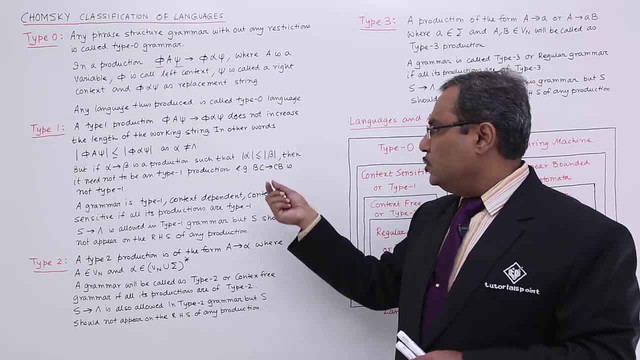 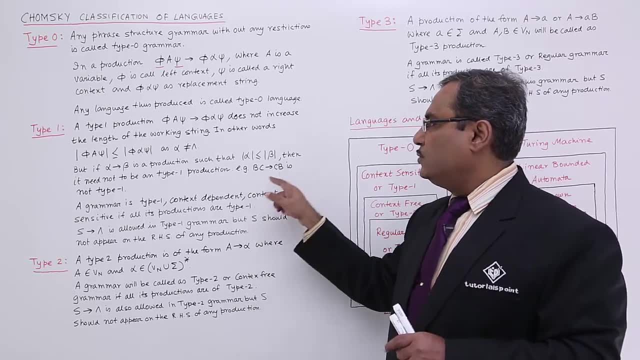 length of CB. Length means what? How many grammar symbols? So here length is 2, here the length is 2.. So 2 is less than equal to 2 is correct. But it is not a valid type 1 production. So the type 1 production will be of the type this, whatever it has been in. 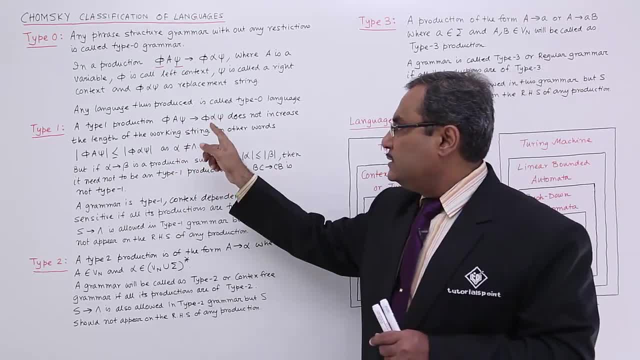 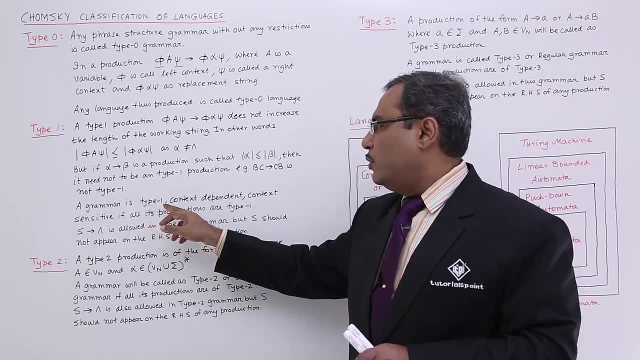 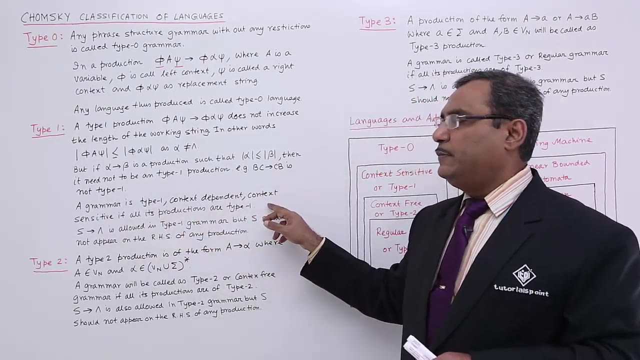 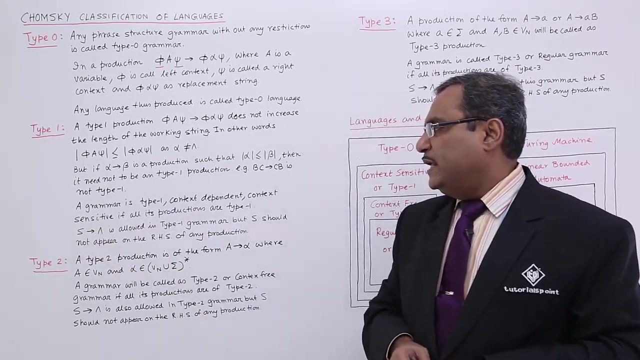 mention And only one constraint in type 1, that is, the length of this must be less than equal to length of this. A grammar is type 1 or context dependent or context sensitive if all its productions are of the type 1.. Starting symbol, say S, produces kappa, is allowed. 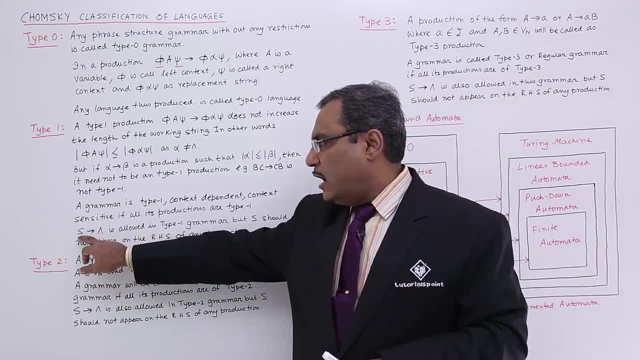 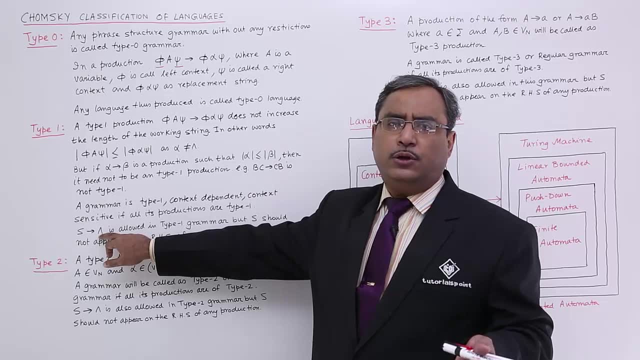 in type 1.. Now see what is the length of S. How many symbols? Only 1.. So length is 1.. And what is the length of this kappa? Length of this null is having the length 0.. So right hand side length is greater than equal to left hand side length. 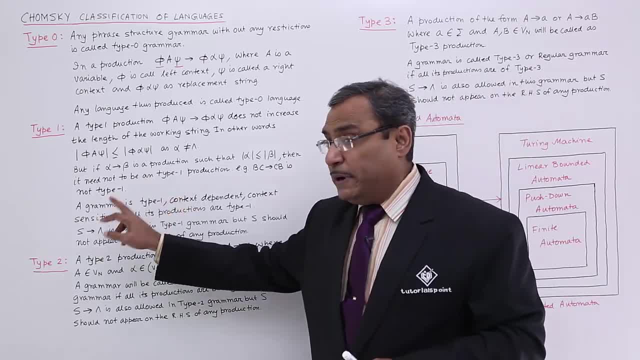 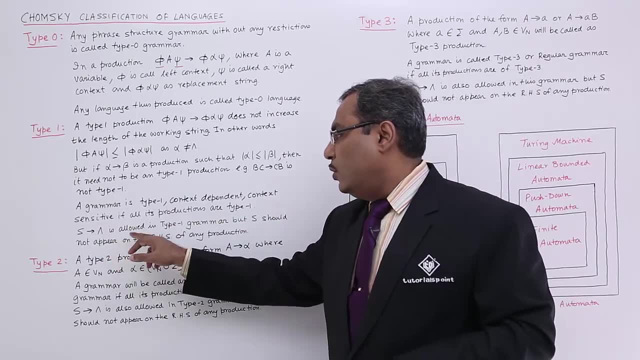 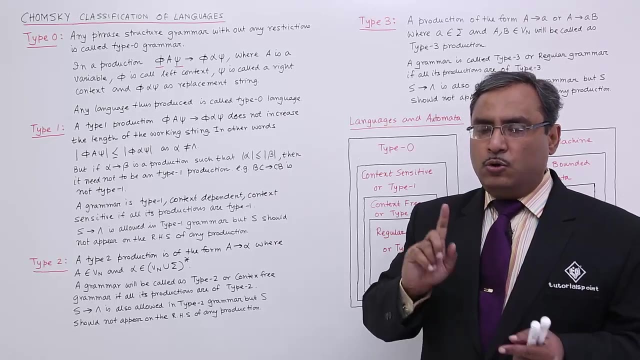 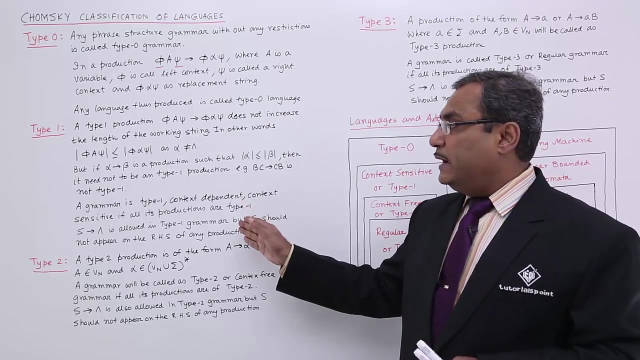 is valid here? No, But in spite of that, S produces kappa is allowed in type 1 grammar, But S should not appear on the right hand side of any production. So that is the relaxation, only for S produces kappa, with one constraint. So that is my type 1 grammar, And the language thus produced will be known as type 1 language. 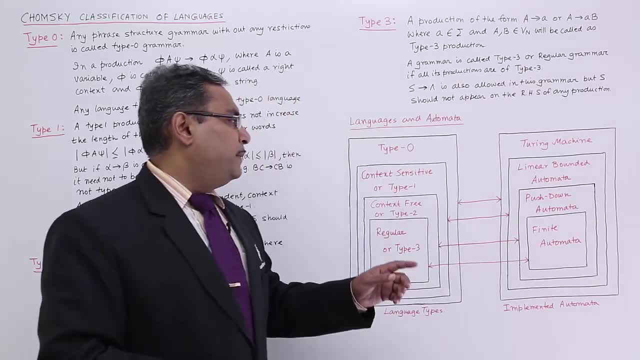 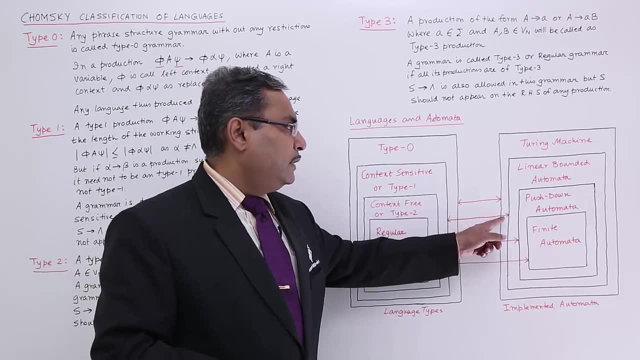 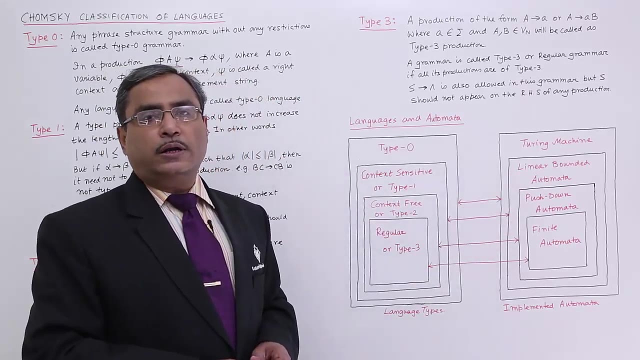 or context sensitive language. So now this is my type 1, which is a subset of type 0. And this type 1 is having the implementation of this is my linear bounded automata. So this type 1 is having the implemented automata is linear bounded automata. 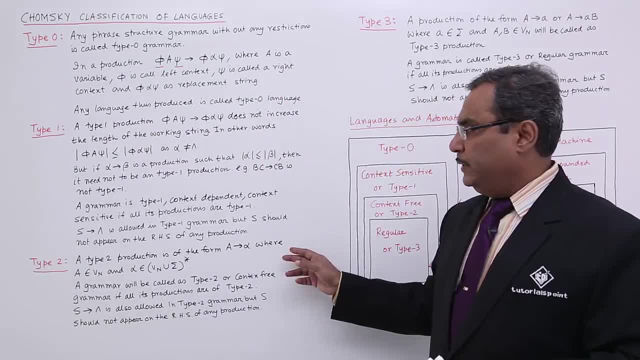 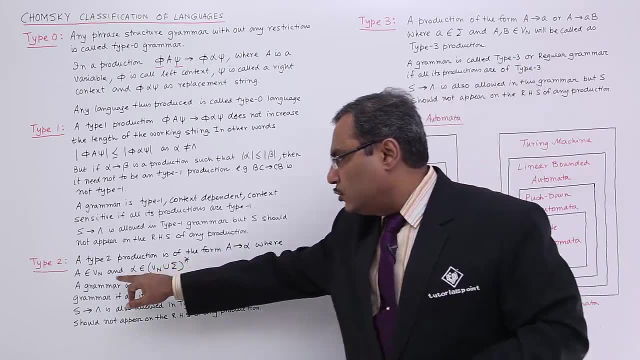 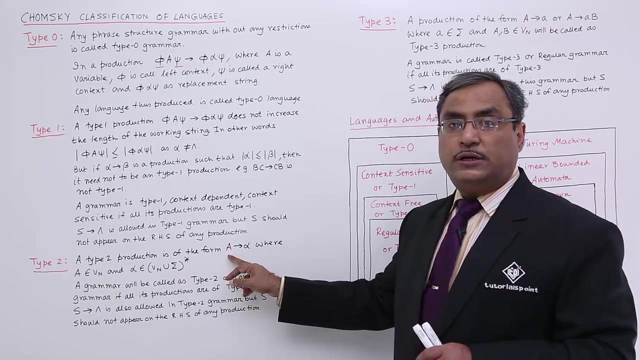 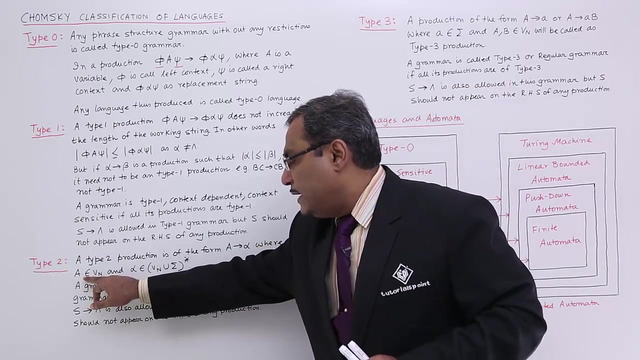 Ok, Next one, my type 2.. A type 2 production is of the form: A produces alpha where A belongs to V? n. See, it is not V n star, it is belongs to V? n. That means on the left hand side of this production we will be having only a single non terminal where and A is belonging to. 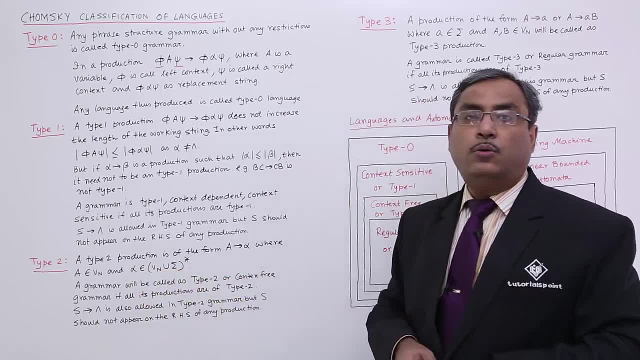 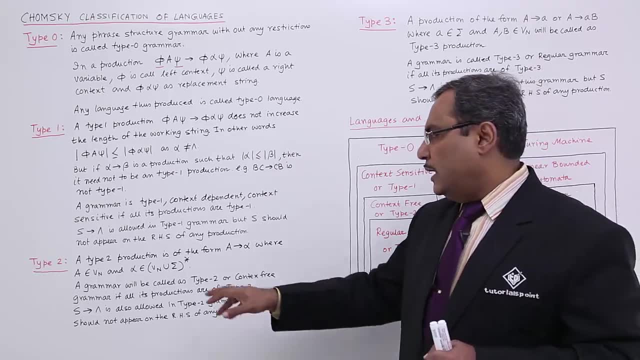 V n and alpha belongs to V n, union sigma whole star. That means on the right hand side it can. it can be a combination of terminals and non terminals. So that is not an issue and that is why it is called type 2 productions And always remember type 2 productions are. 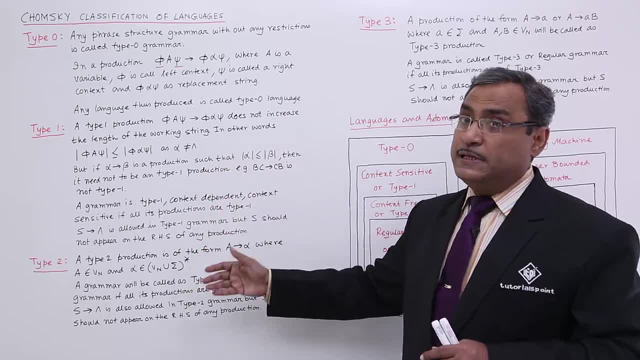 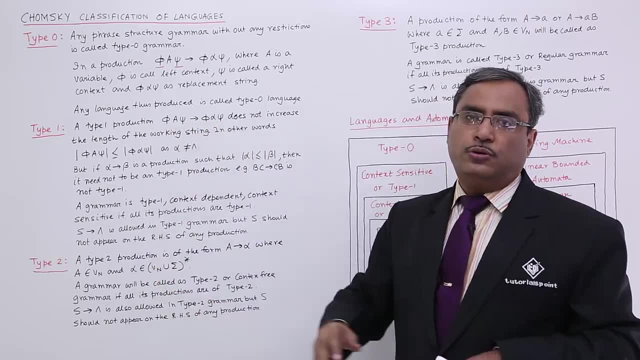 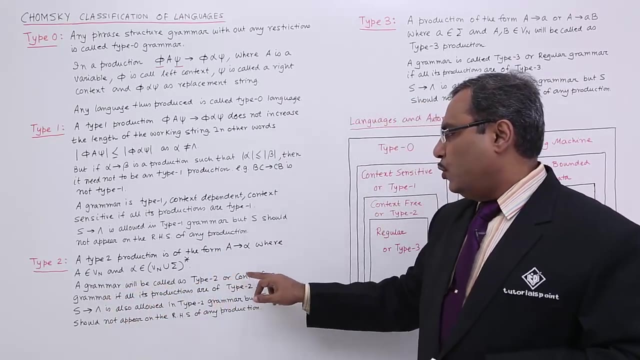 type 1 also. That means it is a subset of that. That means here also that constraint, that is, the length of the right hand side must be greater than equal to length of the left hand side, for each production will be also applicable. Ok, So we have done up to this. A grammar will be called as type 2 or context free grammar. 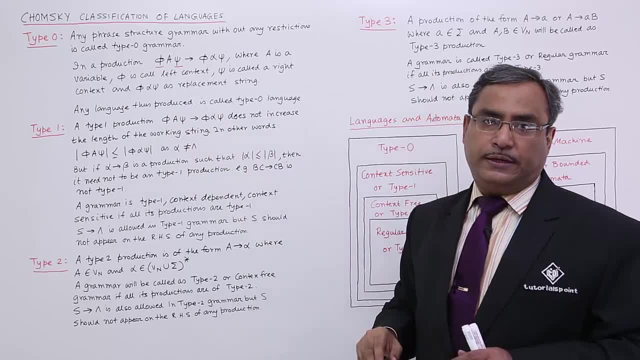 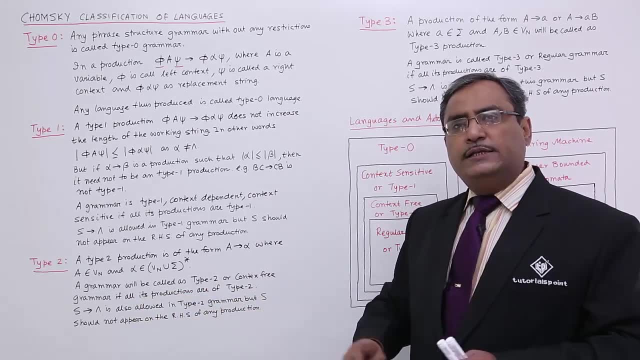 Context free because we are not having any context concept here. So context free grammar if all its productions are of type 2.. If all the productions of a grammar is of the type 2, then the grammar will be known as the type 2 grammar and or context free grammar. and 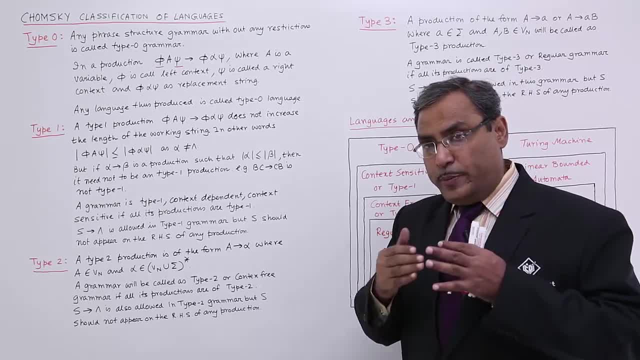 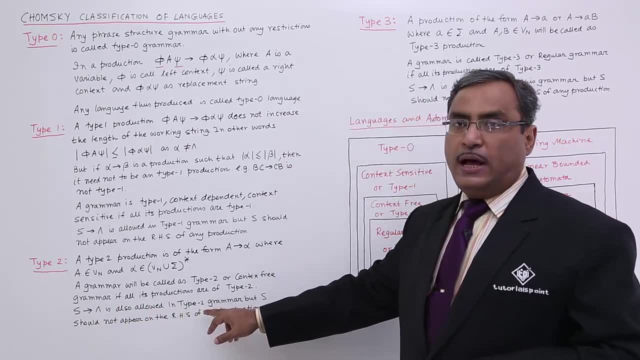 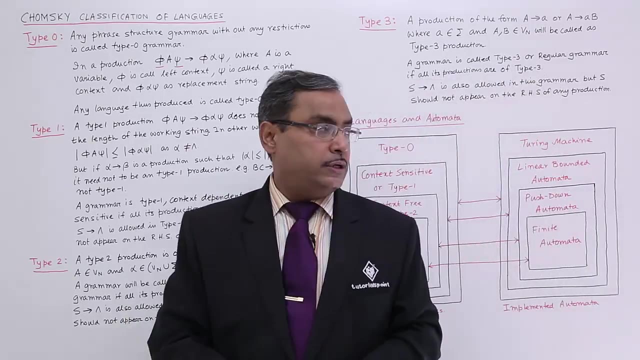 the language thus generated will be known as context free language or type 2 language. S produces kappa is also allowed in type 2, as it was allowed in type 1 grammar, But A s should not appear on the right hand side of any production. So that is my type 2. that. 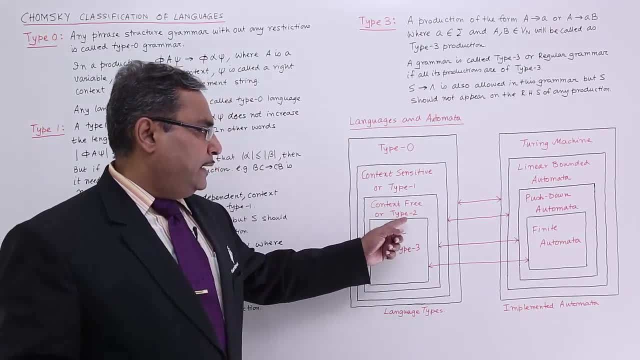 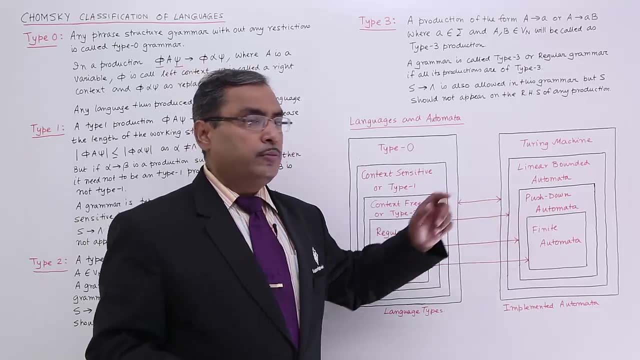 is a context free or type 2 language and it it is having the implementation of this, my, this, my pushdown automata. So it is having the implementation of pushdown automata. And what is pushdown automata? We will be having series of videos on the pushdown automata. 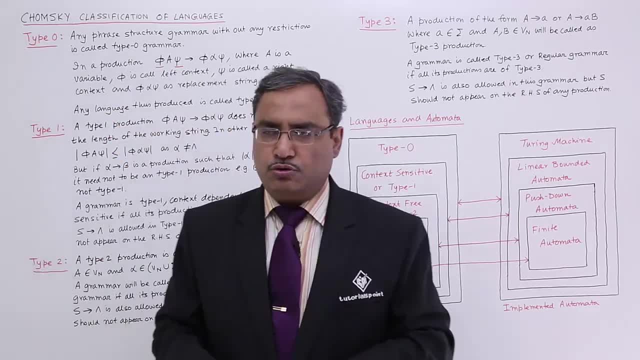 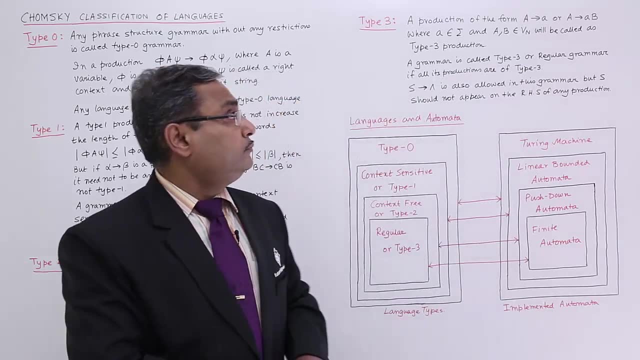 and the respective get question, paper, solve and all you can easily go through them. So we have completed type 0, type 1, type 2.. Now let us come for type 3. A production of the form capital A produces small a or. 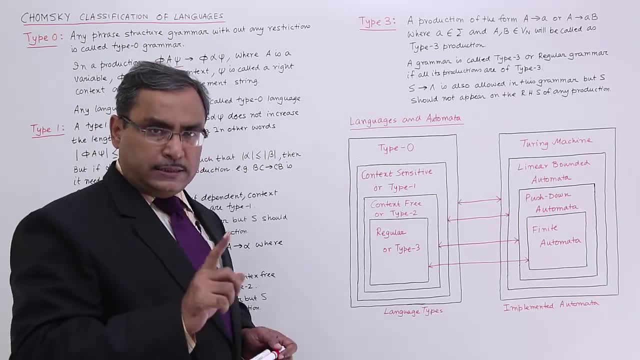 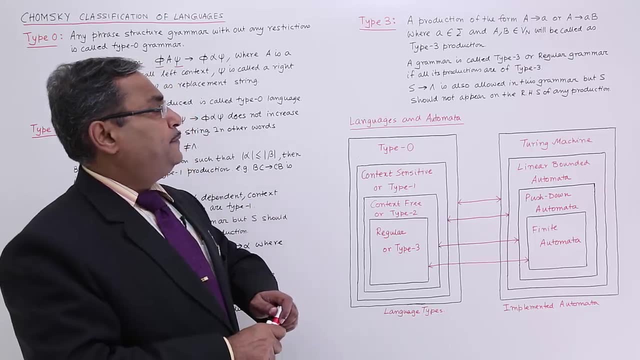 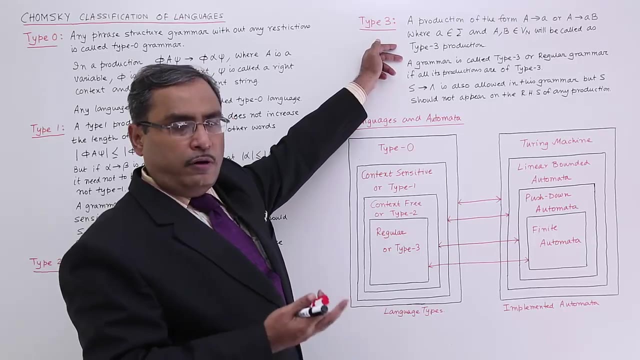 capital A produces small a. capital B, That means non terminal produces terminal, or non terminal produces terminal, non terminal, If such productions are existing and where small a belongs to sigma. obviously that is the set of input alphabets or set of terminal symbols. rather, I should say: 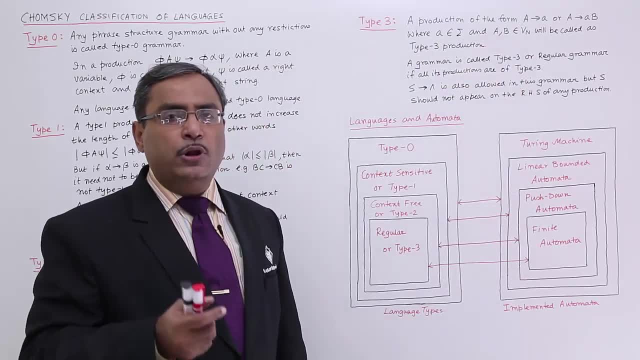 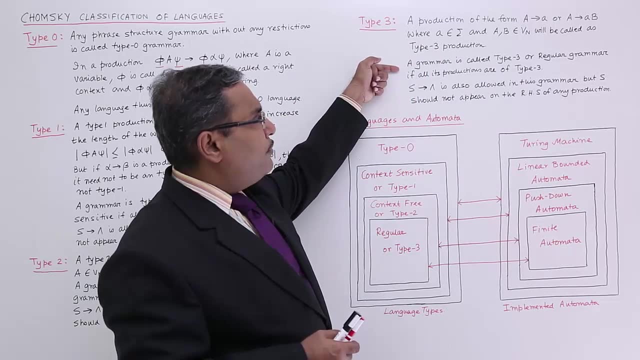 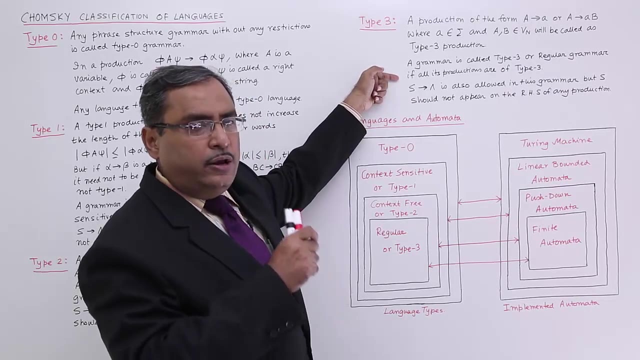 And A and B are nothing but a non terminal symbols, So they will be belonging to V. n will be called as type 3 productions. A grammar is called type 3 or regular grammar if all its productions are of the type type 3.. And whenever type 3 productions are there, they 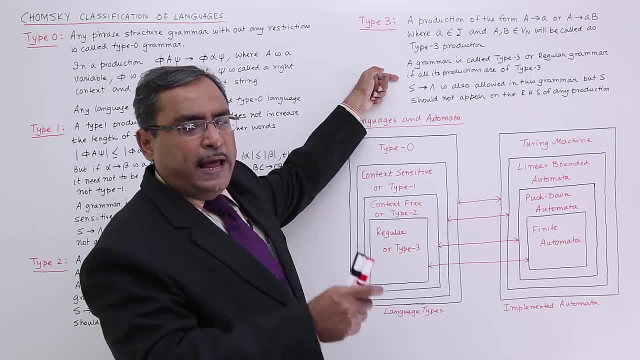 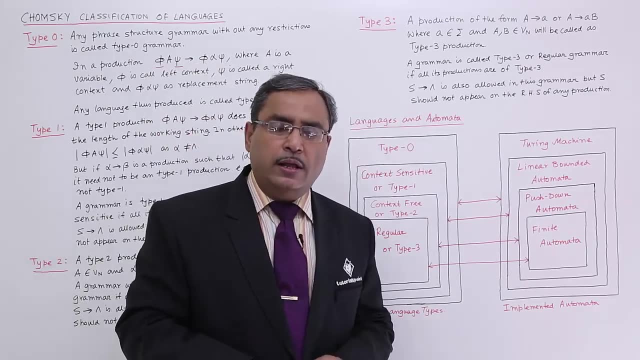 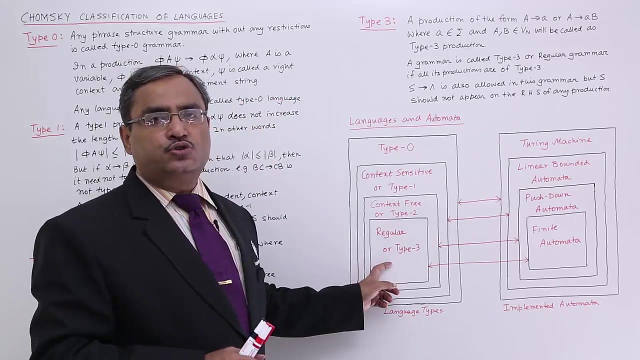 will produce a grammar called regular grammar and the respective language will be called as regular language or type 3 language. S produces kappa is also allowed in this grammar, but S should not appear, But on the right hand side of any production. So now that is my type 3, that is the innermost one. It is a subset of this, this context free. 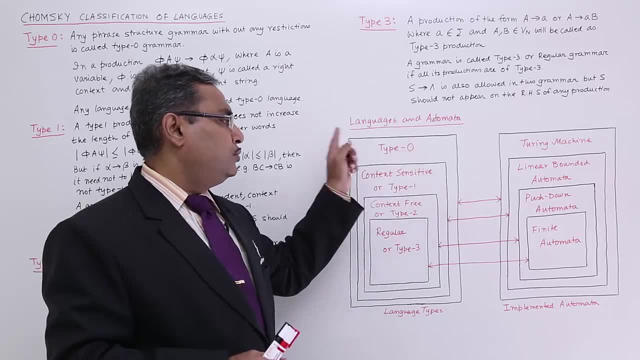 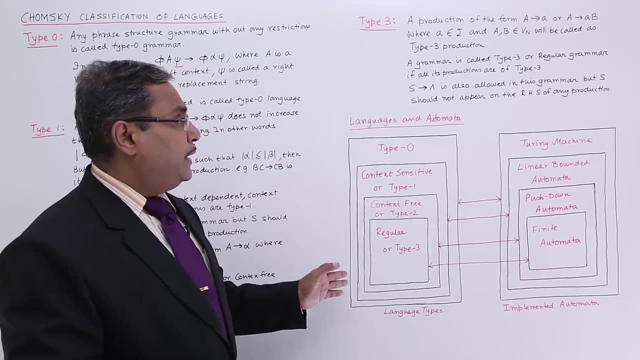 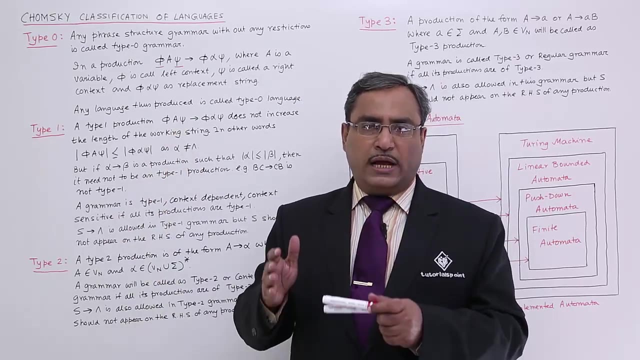 or type 2 subset of type 1, and type 1 is a subset of type 0. So the diagram has been drawn accordingly and it is having the implementation of finite automata. So in this way the classification of languages can be done in between type 0, type 1, type 2 and type 3.. I think you have. 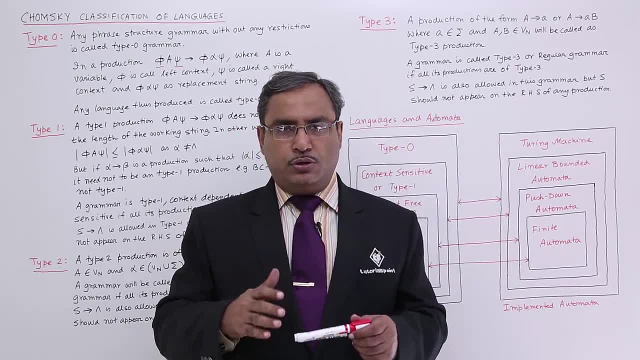 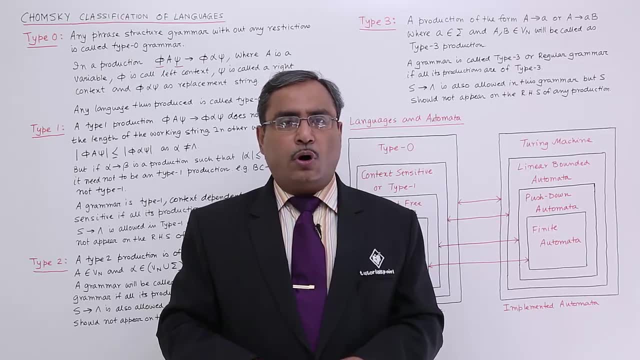 got, got my logic how the type 0 to type 3 language types have got classified and in this way will be also solving problems on this particular topic. Thanks for watching this video.